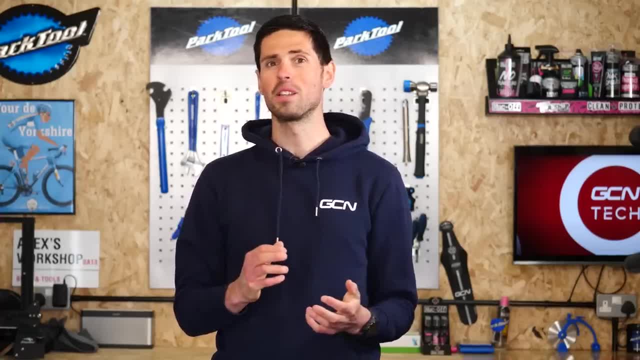 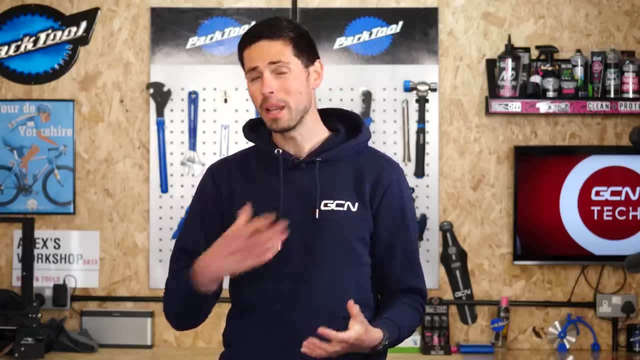 Now, then, I've got something a little bit different in store for Maintenance Monday this week, because we're going to start a mini-series, a crash course as such, in road bike maintenance, taking you from complete beginner through to more competent home bike mechanic To help guide us. 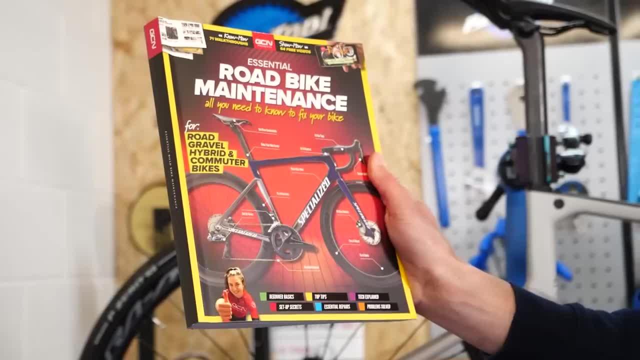 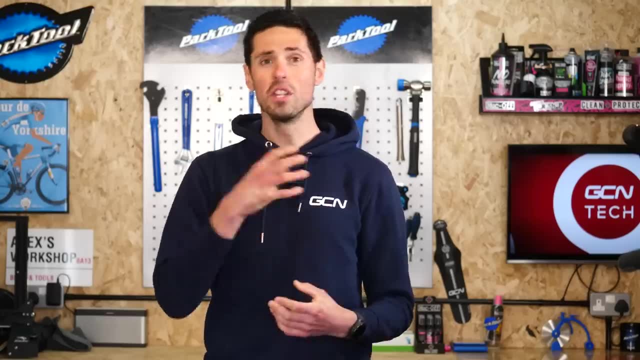 along the way, we're going to be referencing the GCN Road Bike Maintenance book. Don't worry, it's not a requirement. so let's get into week one. We're going to be taking a look at some of the basic principles and knowledge to help stand you in good stead for the future Along the way. 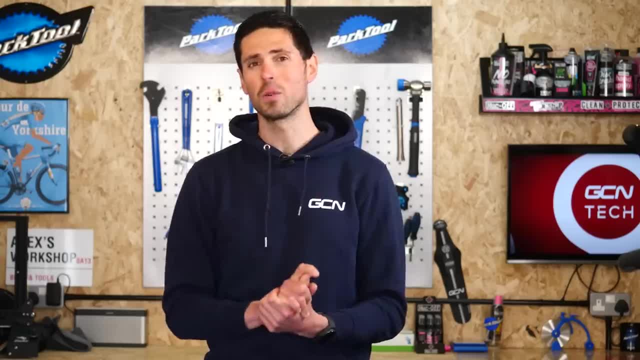 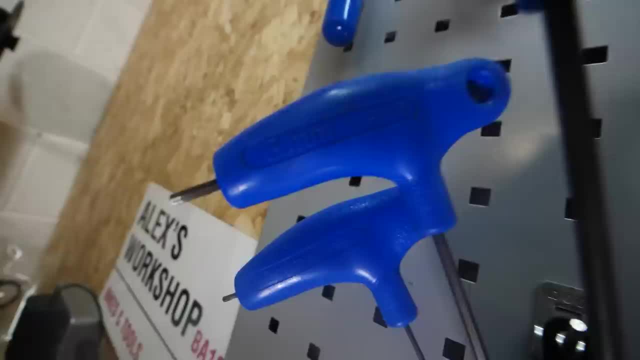 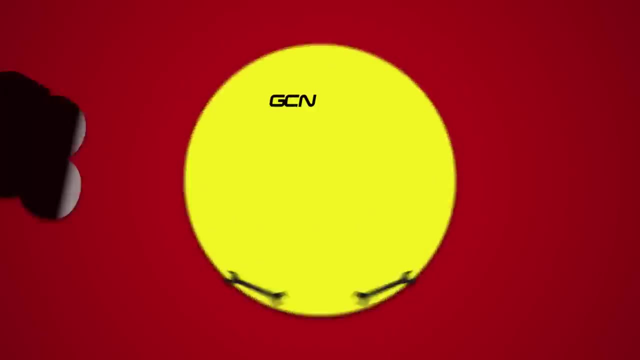 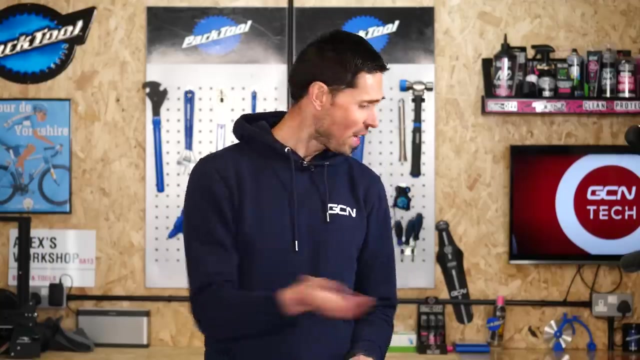 we're going to look at some simple maintenance tasks that will help keep your bike running sweet, mile after mile or kilometer after kilometer. Right then, it's week one. What are we going to be doing? First up, we're going to take a look at 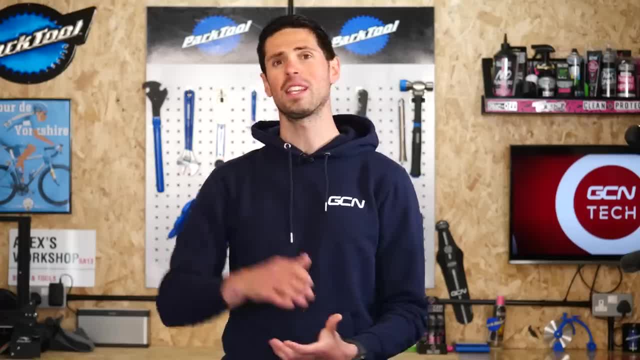 some of the components on our bikes and what it is they do. Then we're going to take a look at some of the components on our bikes and what it is they do. Then we're going to take a look at some basic tools that we're going to use as we progress through the weeks. Don't worry. 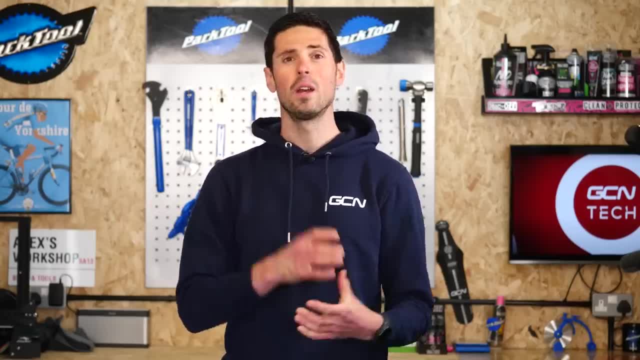 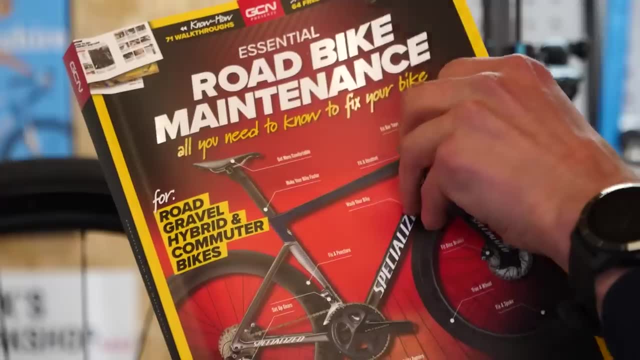 you don't need to rush out and buy the most expensive tools you can. We're going to be using the sort of stuff that you might have just lying around at home. If not, they can be picked up for a nice, reasonable price If you turn to page 18 of your essential road bike maintenance books. 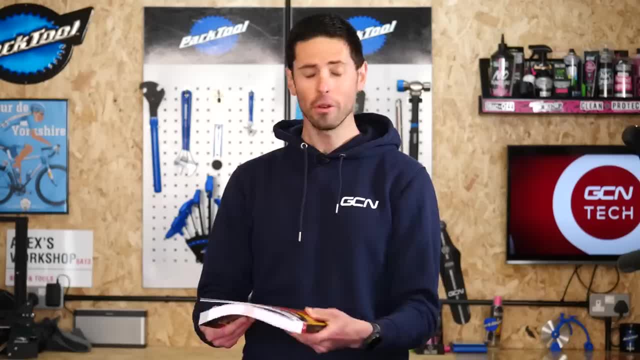 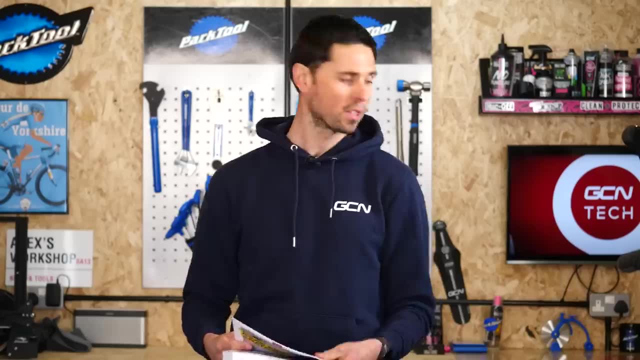 you'll see the anatomy of a road bike. I never thought I'd be saying that. I sound just like a school teacher. but don't worry, we're not going to run through exactly the same list as what we've got in our books. We're going to take a look at our bikes and give a brief explanation. 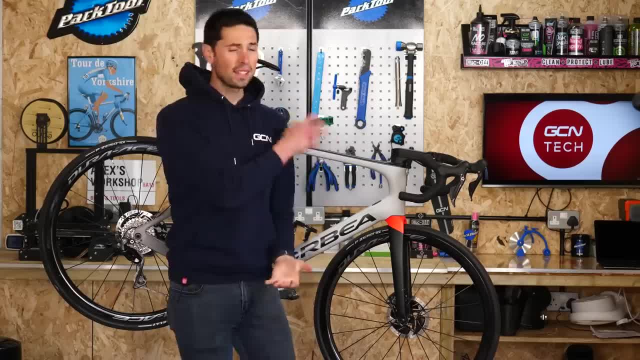 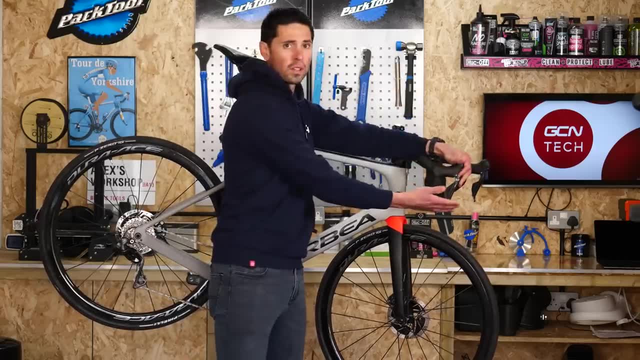 of what some of the components do. Let's take a look at some of the components on our bike, Starting at the front. what better place to start Up? here we've got what's known as our shifters. These allow us to pull the brake, to apply the brake force through to the wheel and also allow 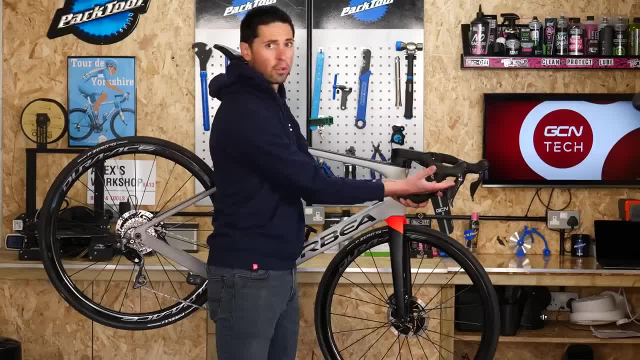 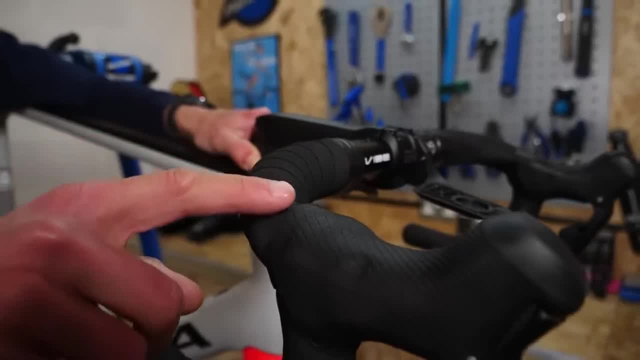 us to change gear with the little buttons here. These are Di2, so electronic shifting, but there is also mechanical shifting options available too. We've got handlebars with a handlebar tape. that's fairly self-explanatory. Then here we've got what's known as the stem on our bikes. This 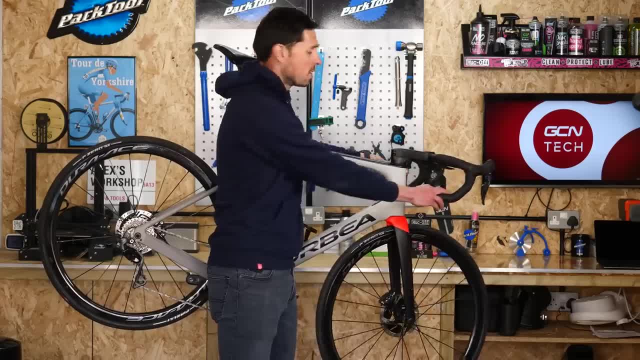 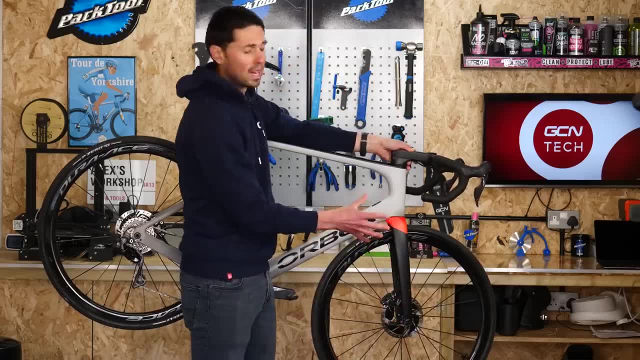 connects the handlebars through to the forks and allow us to turn securely on the bike. The steerer of our forks runs all the way down through here and these are the forks which the front wheel is attached to. You can see down here. we've got a disc brake bike. We've got a disc brake. 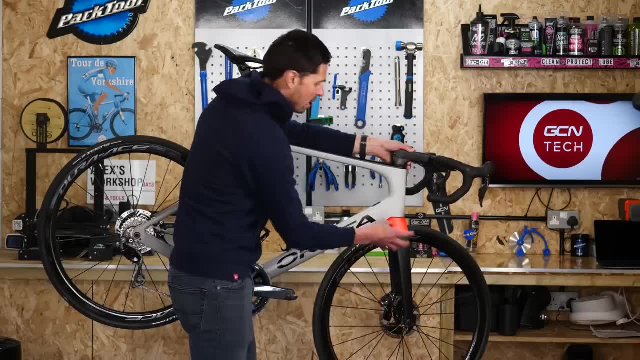 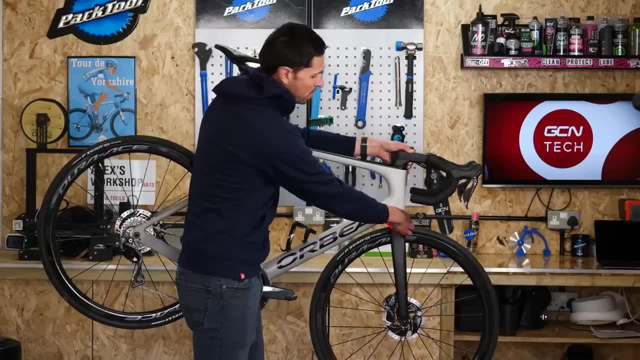 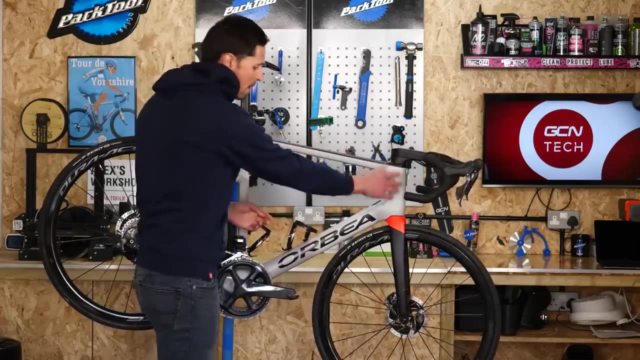 caliper and the rotor that the braking surface is housed onto. You could also get a rim brake bike caliper on the front of the forks here and then a braking surface all the way around the wheel. That's the other braking option that's available. These are the main tubes of our frame We've got. 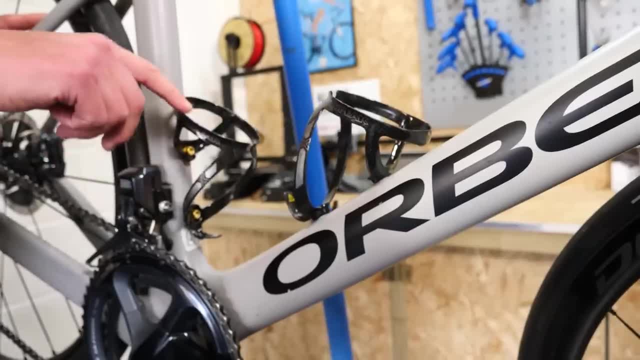 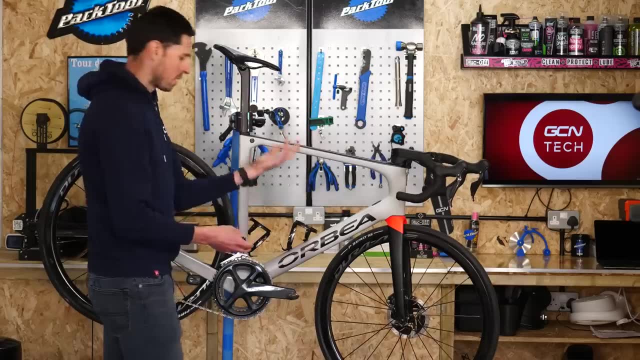 the top tube along here and the down tube here, As you can also see. we've got our bottle cages here where we can store certain parts and spares that we might take out on the ride, as well as our drinks. Coming to the center of the bike down here. we've got our chain set. 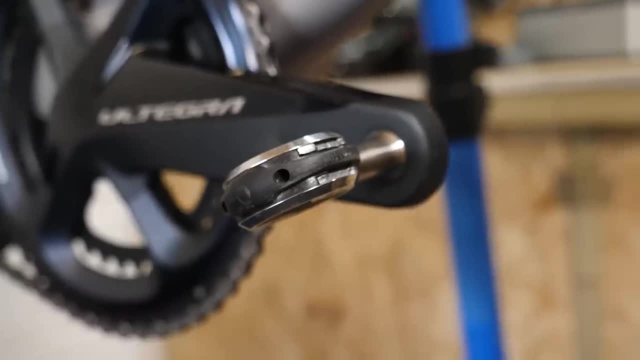 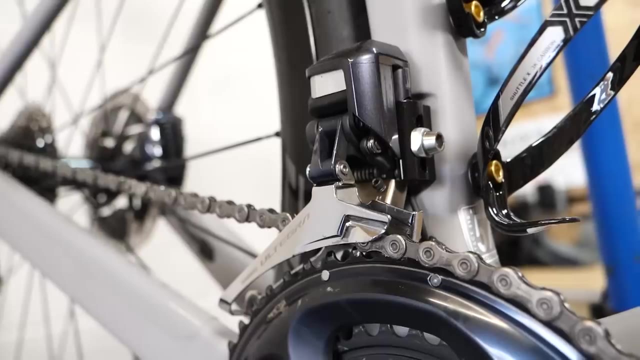 This also features the pedals, and this allows us to transfer our efforts in the bike forwards. This chain set has two chain rings on it. This is changed by the front derailleur here, which guides the chain over the different chain rings. There's also the option of 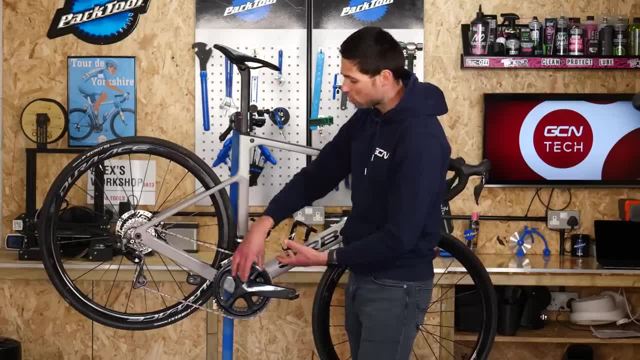 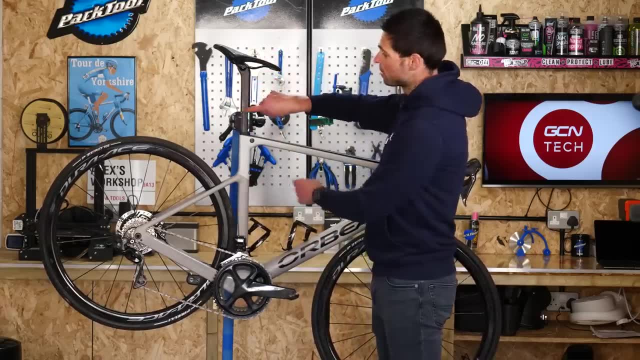 having a single chain ring, or some bikes might even feature a triple chain ring option, and that just gives a far wider range of gears Coming up. here we've got the seat post of our bike, and this can slide within the frame or extend further up so that we can adjust the bike to fit. 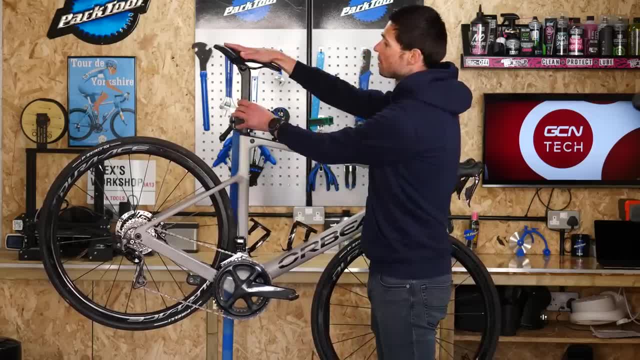 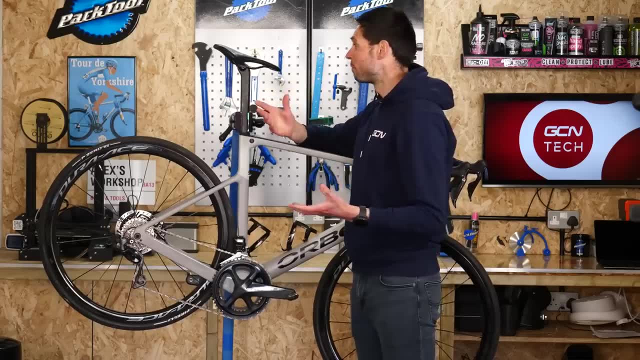 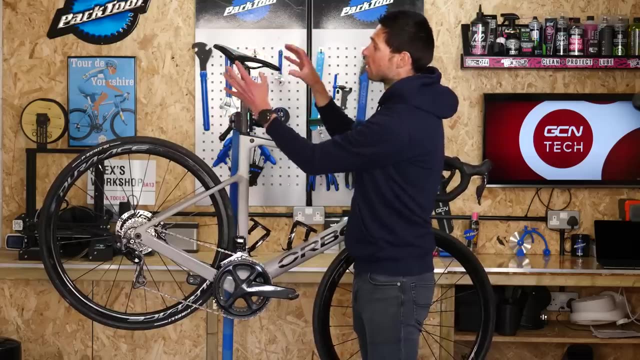 a different variety of size riders. Right at the top of the seat post is our saddle. There are loads of different types and sizes of saddles available to suit as many different riding styles as you could possibly imagine. This is adjustable forwards and backwards, and you can also adjust the angle this sits at as well. 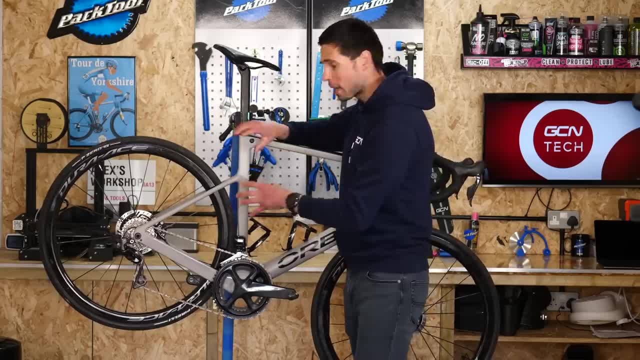 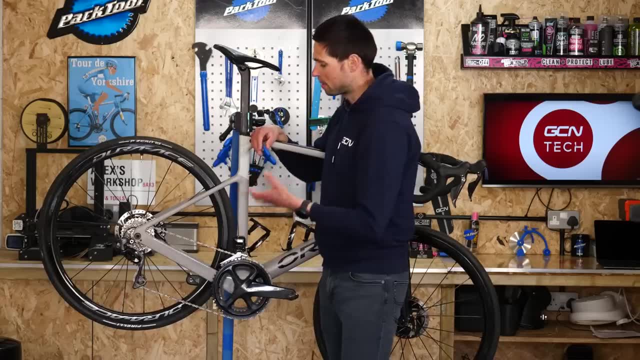 to make sure we're nice and comfy on our bikes. Moving to the back of the bike, this is our rear wheel. We've got the valve here, which is used to pump up our tires and ensure they're inflated to the correct pressure. We've got a chain that runs all the way around. 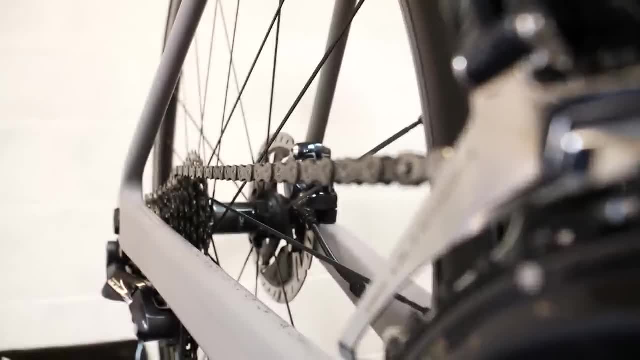 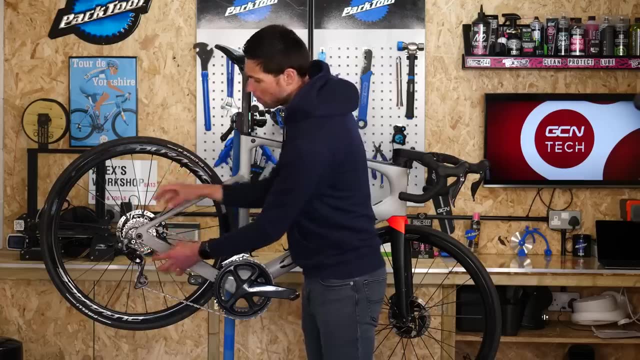 here, and that is to take our efforts from our chain set at the front to the rear wheel and drive the bike forwards. Also at the rear of our bike, here in the center of the wheel, we've got what's known as the rear derailleur, which some people might call the rear mech. This is used to guide. 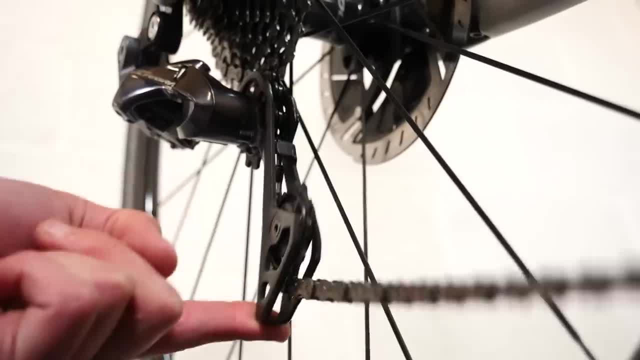 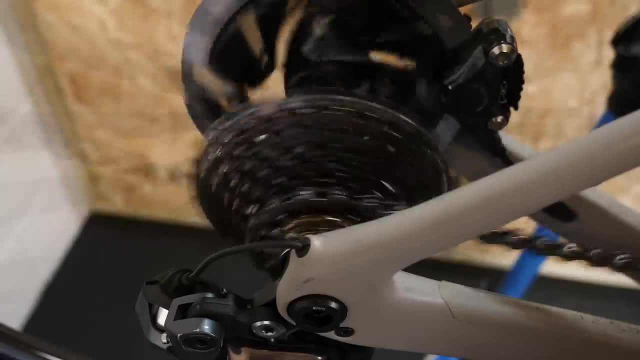 the chain, apply some tension to it, as you can see here with a spring, hold the chain nice and securely on the bike. Then it also guides the chain across the different gears on our cassette. The cassette is this part here with all of these different teeth. 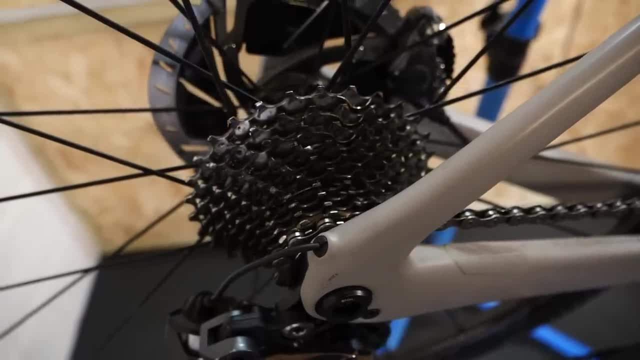 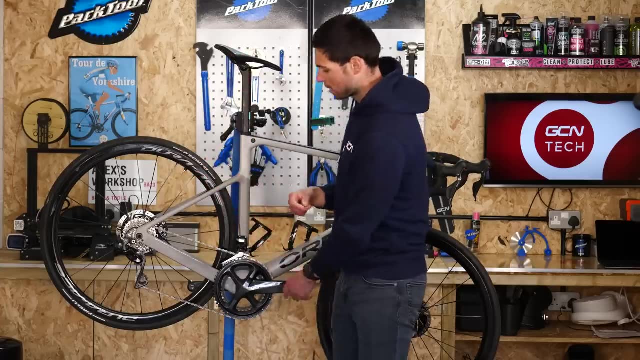 and size sprockets on it, allowing us to change the gear ratio of our bike depending on whether we're riding uphill or downhill, enabling us to ride at a comfortable cadence. Our cadence is our pedaling rate, so the speed that these cranks are turning at. 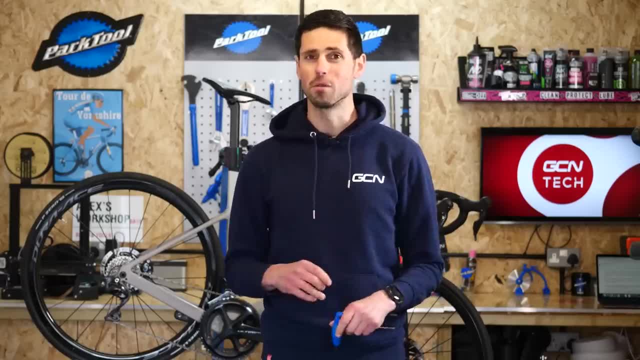 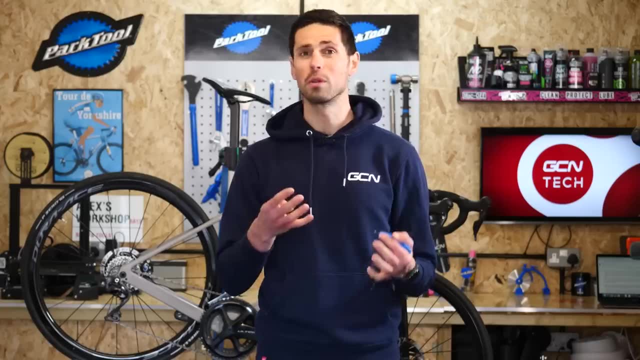 Those are some of the common parts on our bikes, but what about the tools? Well over on page 24 and page 25 of our road bike maintenance book are some perfect examples of the tools we'll use when our bikes. One of the most common tools we're going to use are our hex keys or Allen keys. 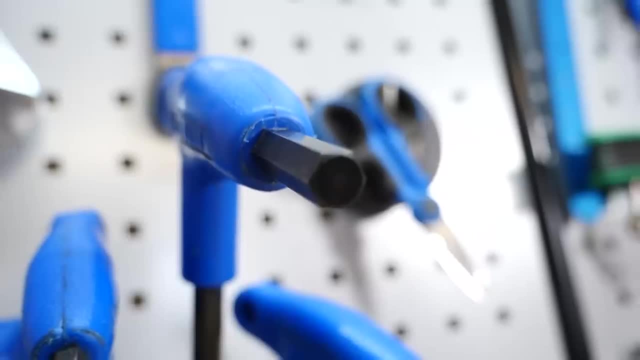 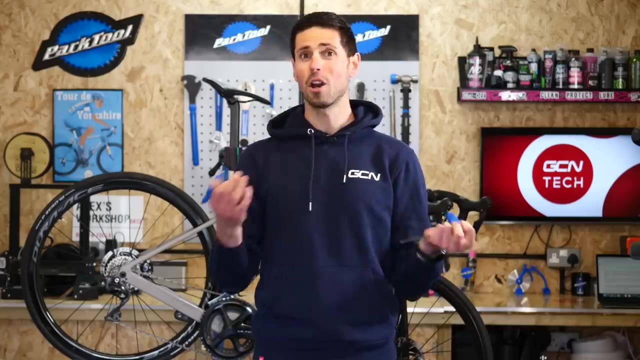 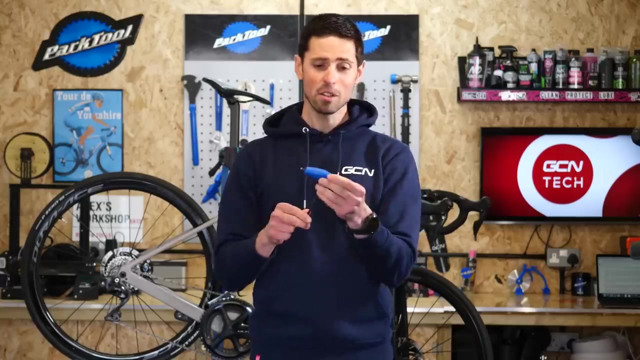 as they're sometimes referred to. As the name suggests, these are in hexagonal shape, which fits into an opposing hexagonal-shaped hole on the bolts of our bikes. The most common sizes that we'll see range from about a 2-millimeter up to a 10-millimeter in size, Depending on the level. 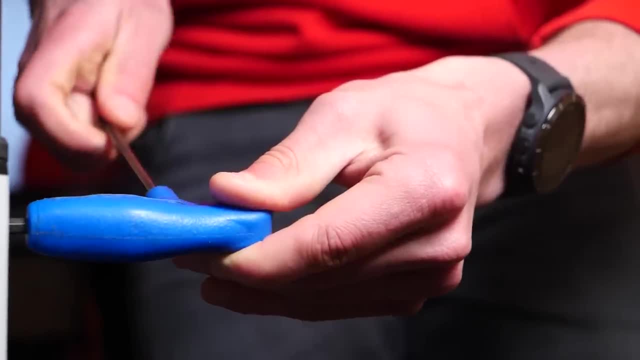 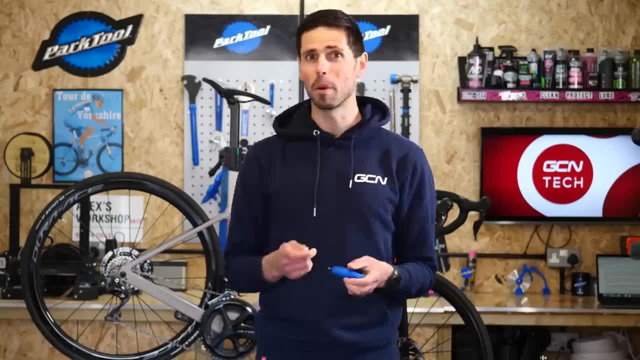 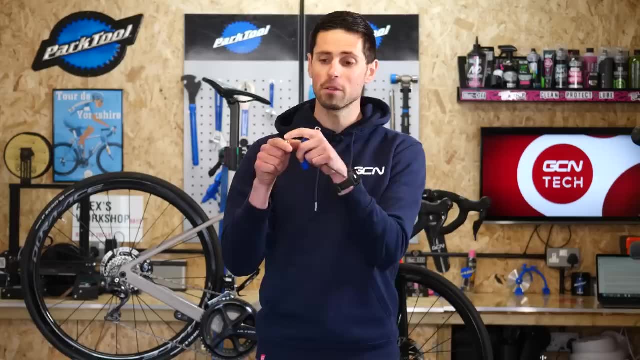 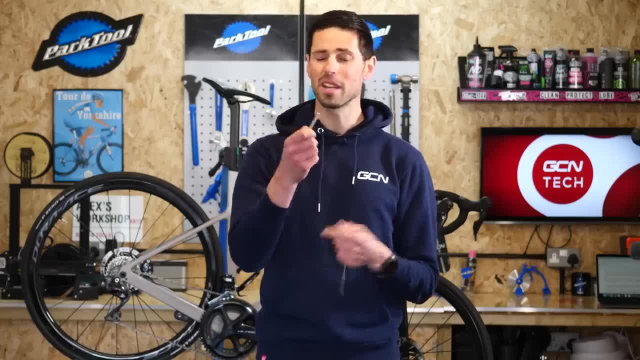 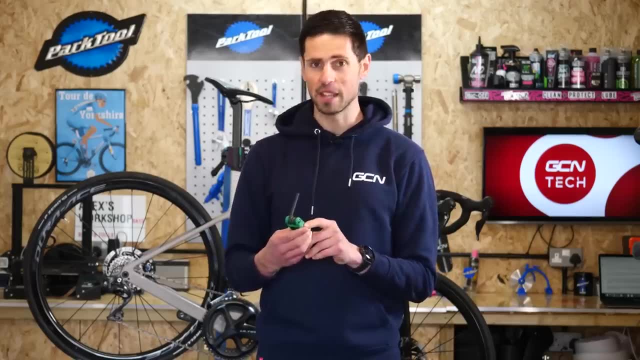 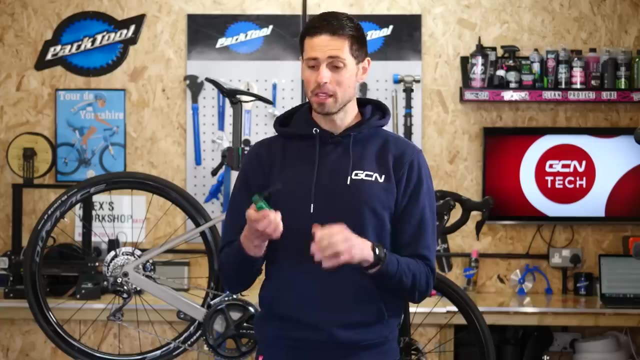 holes and make it incredibly difficult to remove the bolts of your bike. No one wants that headache. Next up are Torx keys. These are an alternative bolt interface to what we have in a hex key. These feature a six-point star shape in a similar design to a hex key. but you've got to remember. 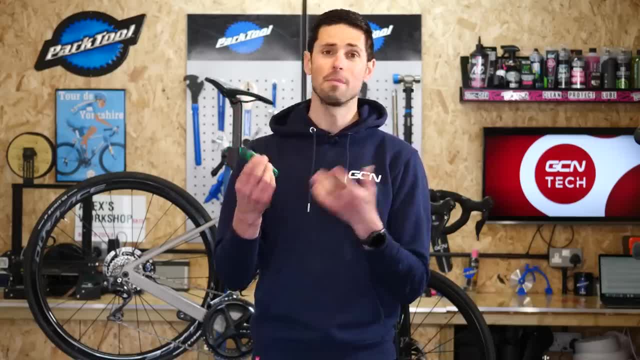 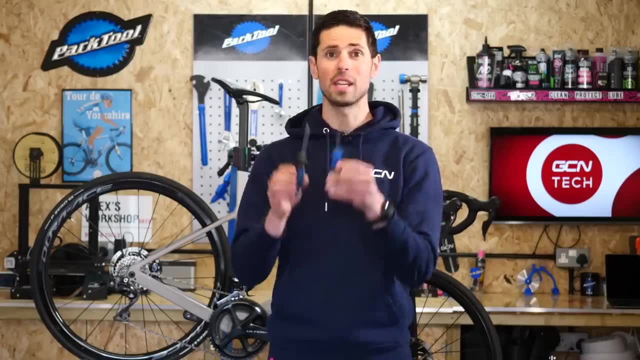 these are not interchangeable. Depending on what bike you've got, you may well have a mix of hex and Torx bolts on it Onto our final tools for week one of our maintenance crash course. taking a look at screwdrivers First up, what you need to know. there are three different types of screwdriver. 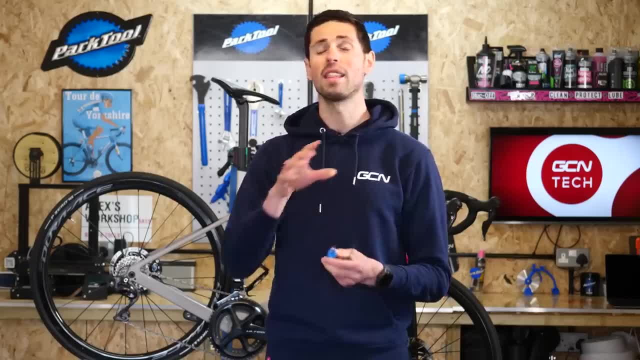 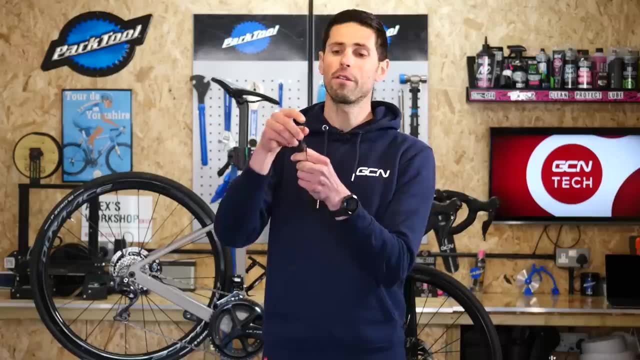 interfaces, starting with Phillips or PosiDrive. The difference between these is quite subtle and you can see that on our handy little on-screen graphics. Next up, you've got your flat-headed screwdriver. Again, we've got a little graphic for that It's.